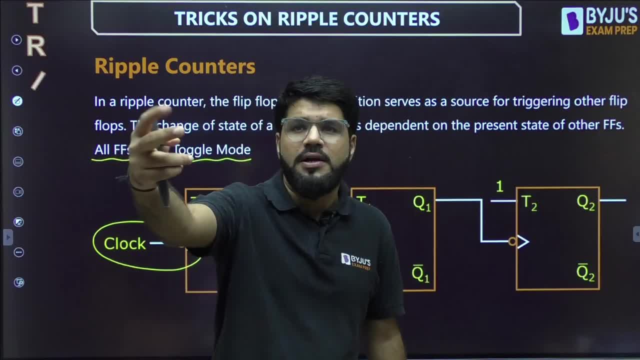 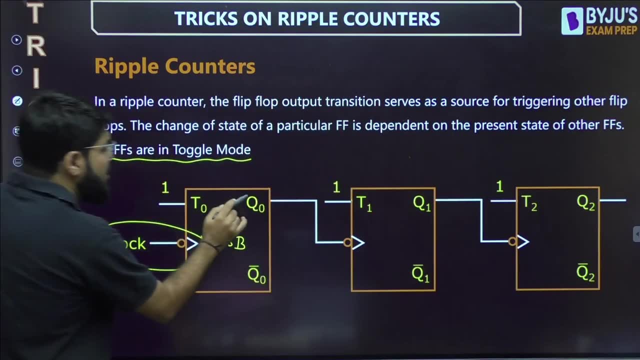 equal to 1, because when t equal to 1, the next state will be toggled, complemented. Similarly, if you are designing using a jk flip-flop, both j and k equal to 1 for the toggle mode for the complement state, and then the output of a flip-flop goes to the next clock, The output of the flip-flop. 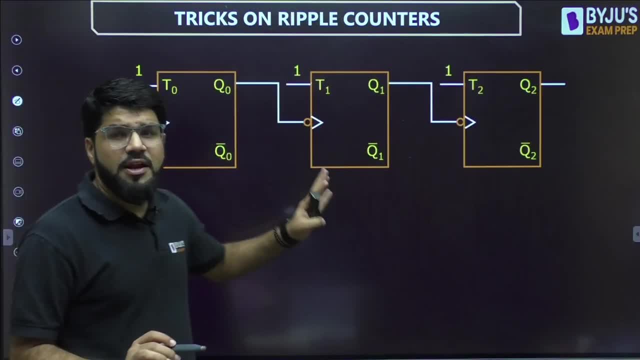 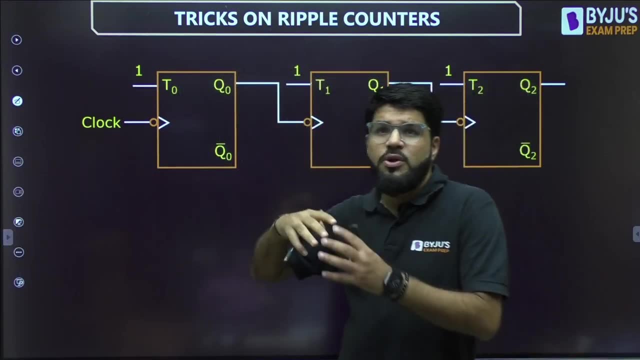 goes to the next clock, and so on and so forth. right Now, normally, we are required to solve this. what is the state, what is the state sequence of this, whether it is up counter or down counter? Yes, we can solve it up because we know how flip-flops. 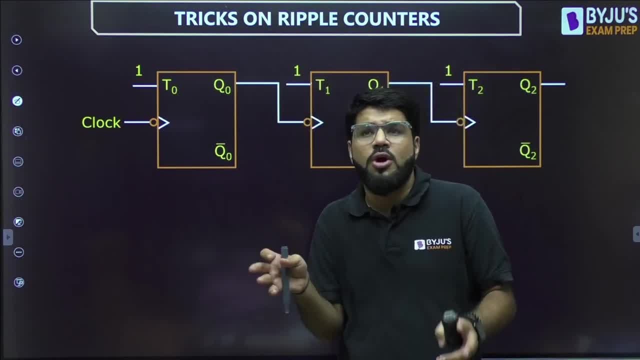 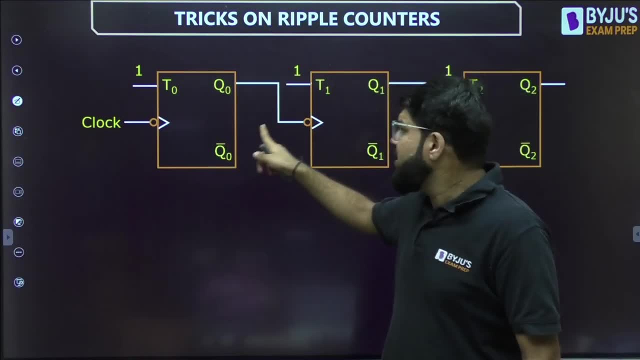 function. what is this? positive or negative edge triggered? but right now we are not here to solve, we are talk about the trick. Okay, and what is the trick? look into the connection, whether the clock connection is from q or q bar, or whether it is a positive edge triggered or negative edge triggered. 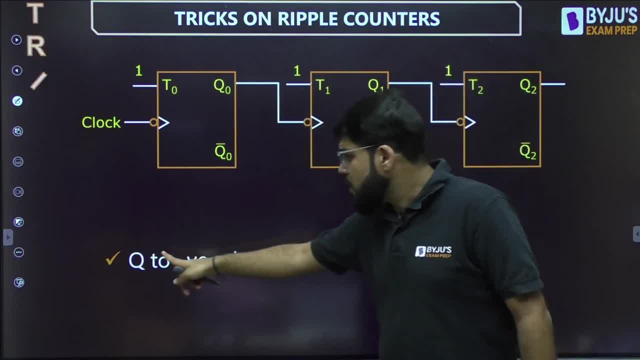 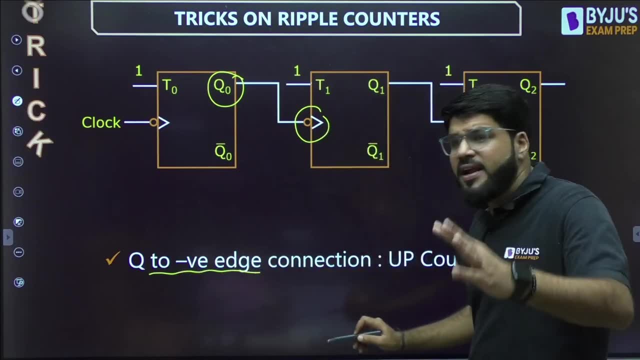 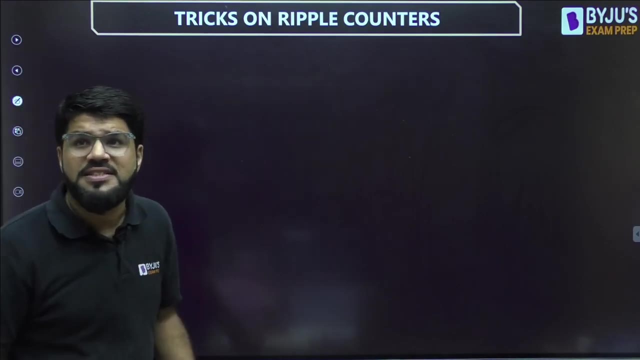 flip-flop. What is the condition here? Here it is q to negative edge. Okay, this is the q output going to negative edge. you take it confirm. confirm, confirm that it is going to be up counter. If it is connection from q output to negative edge, it is up counter. if I change something, if I change something. 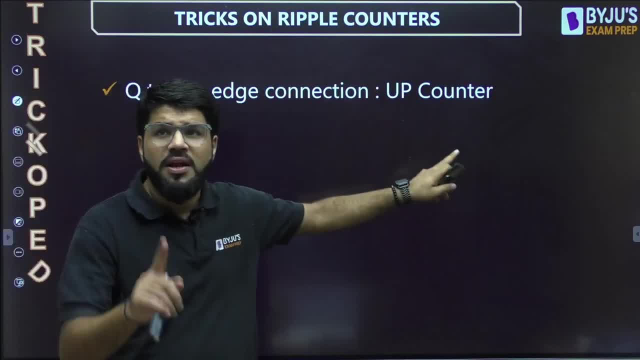 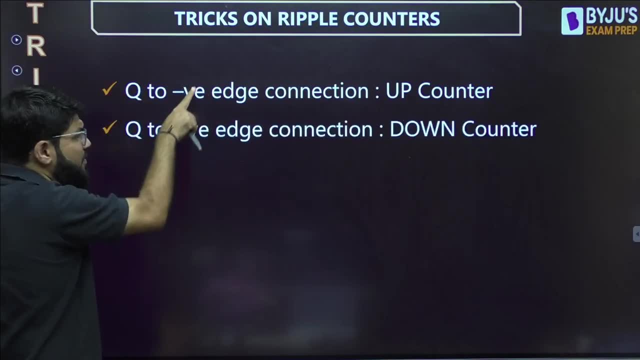 then have a look into this. So that's what, if it is q to negative edge, up counter, if you change any one parameter, it will reverse like up will become down. So rather than q to negative edge, if you take q to positive edge, I have changed one parameter- it should become down. Up ka down, ho jayega right. 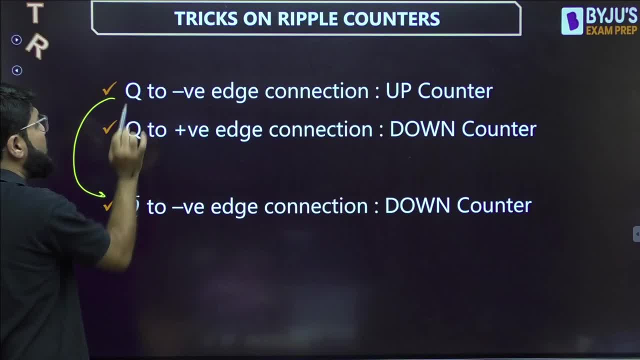 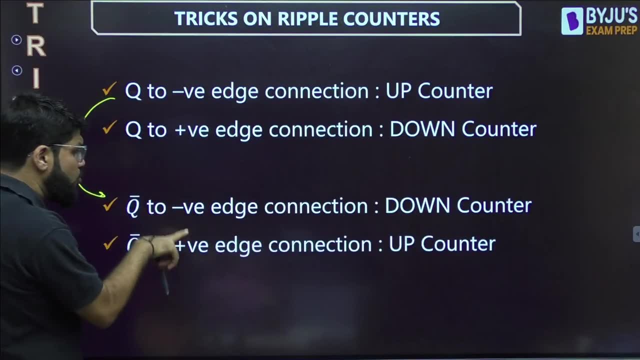 Similarly. look into this now: q to negative. I change one parameter. I may take it as q bar, q bar to negative. one parameter changed, up becomes down. Okay. so similarly, q bar to positive right, q bar to positive: only one parameter change. so again down will become up. That is one of the trick One. 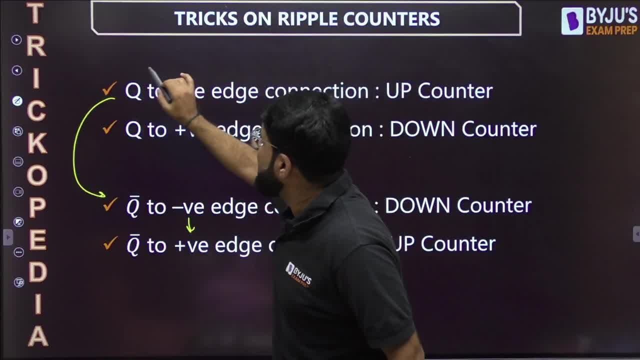 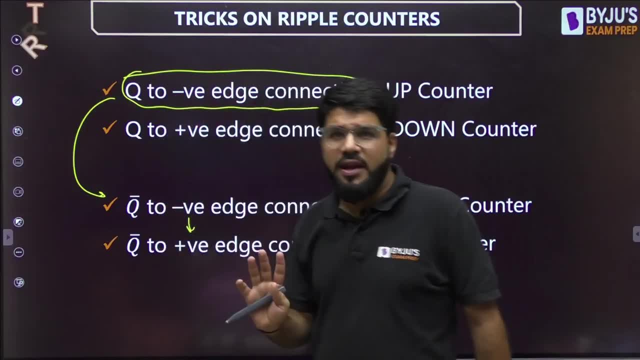 more trick there. I will give you two tricks here. One trick is: just have to remember one type of connection q to negative edge. that is up. If any one parameter change, it becomes down, and etc. One more trick. one more trick is again very simple. let us say q means 1. let us say q bar means 0. let us 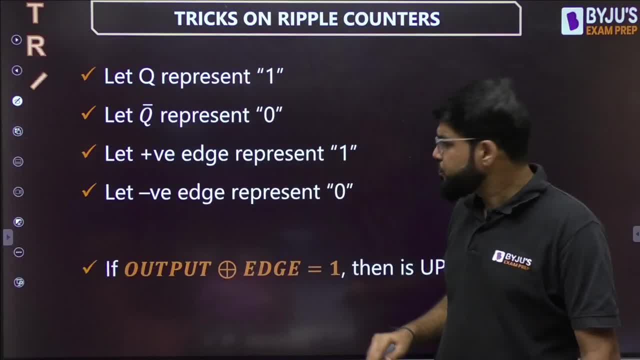 say positive edge is 1, let us say negative edge is 0.. Let us say positive edge is 1, let us say negative edge is equal to 0. right Now, okay, take the output xor edge. okay, and if the output xor edge? that means if they are different, if it gives a one output xor output is i when both the inputs are. 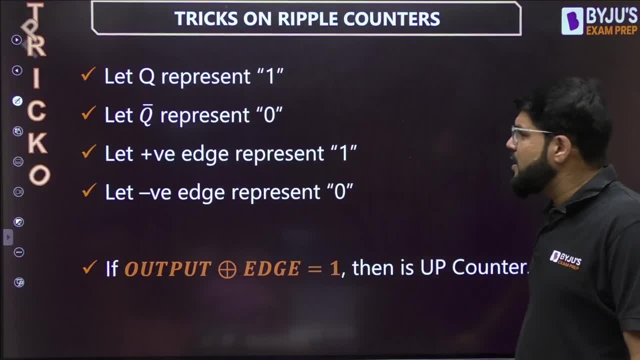 different. So if output and edge is different, okay, then it is always a up counter. Say, for example, q to negative edge: q means 1, right, negative edge means 0. What is one xor, 0 is 1 and what we have seen? q to negative edge is up counter. Okay, that is what you can study. Let us apply this quickly. 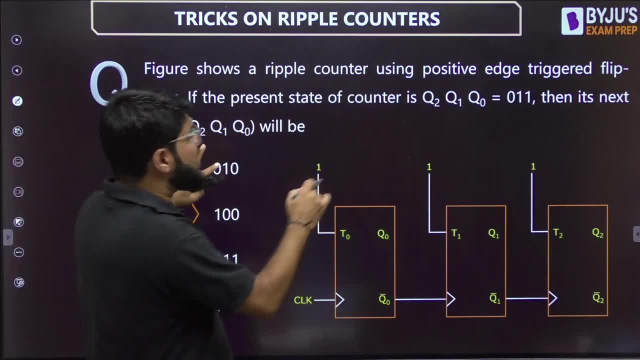 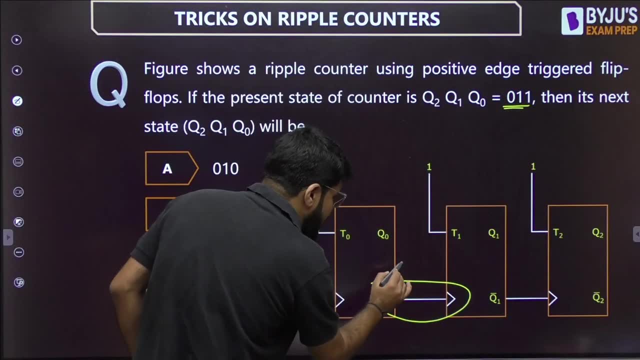 using positive edge triggered flip flop. Okay now, if the present state is 0, 1, 1, what is the next state? very, very simple question, because now look into this connection. What is this q bar, right q bar means 0. What type of edge? positive edge? positive edge means 1, 0, xor. 1 is 1 and if it is 1, it should. 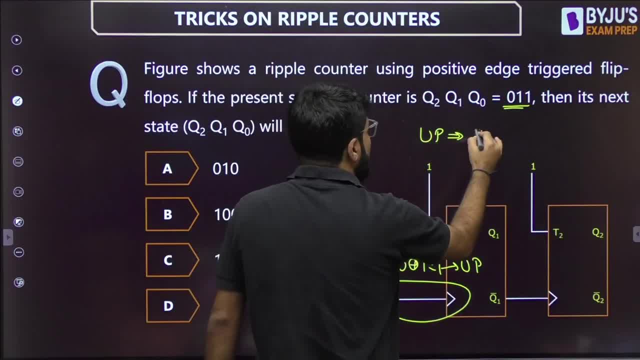 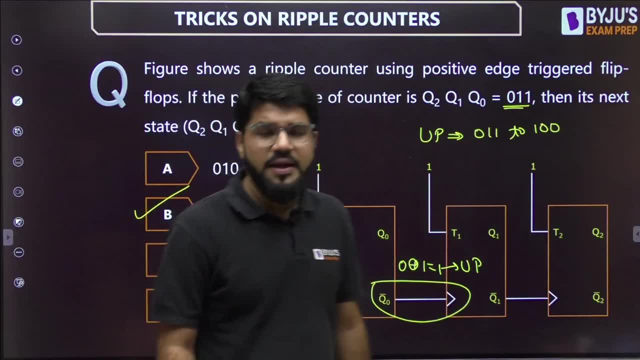 be up counter and if it is up counter, if it is up counter, 0, 1, 1 ke baat. next state: ayega 1 double 0, 3 ke baat ayega 4 na. so correct answer is 1 double 0. the correct answer is 1 double 0.. 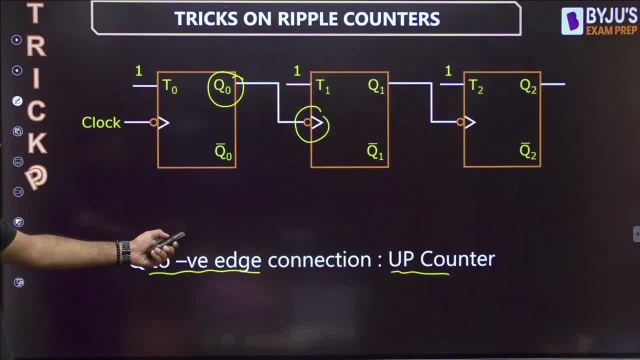 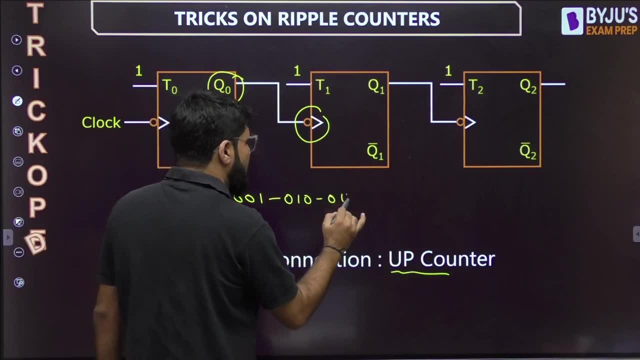 It is up counter, even the counter that i presented. if i go back to that counter, okay, as i told you, it is up counter. so 0 0, 0, 0, 0, 1 0, 1 0, 0, double 1, 1, double 0, 1 0, 1, 1, 1, 1 0, 1, 1, 1 1 and back to 0 0 0. 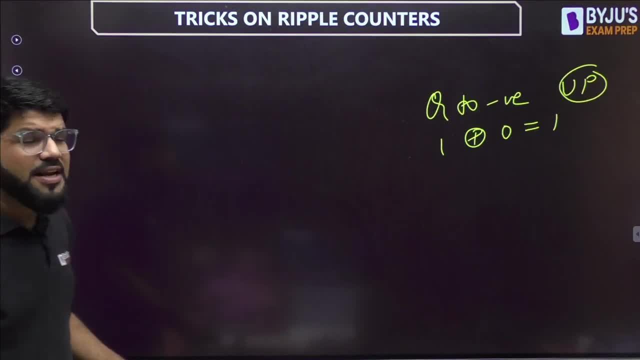 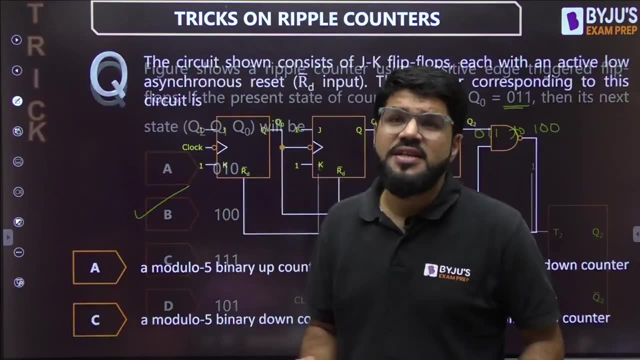 that is what is up. counting is okay. Okay, now let us take another type of very much expected question from ripple counter. usually it is not going to be that simple, but questions are commonly mixed with the concept of reset or the preset pin, which could be mostly asynchronous, but they can. 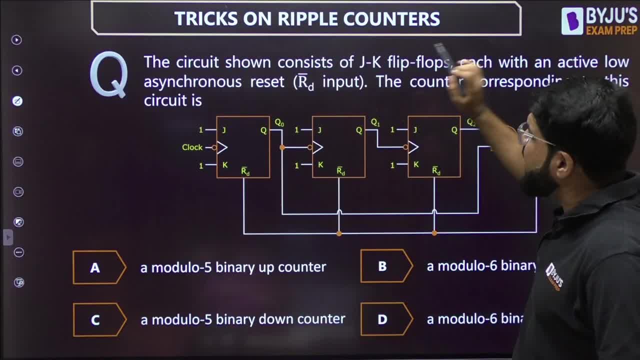 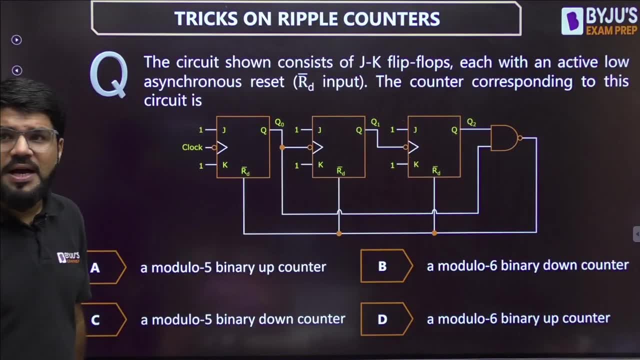 be asynchronous. also, the circuit shown consists of jk flip-flop eat with the active low asynchronous reset pin. the counter is what: modulo 5 up, modulo 6 down, modulo 5 down or modulo 6 up counter? first of all, look into the connection. okay, the connection is of a regular connection that i have taught you. 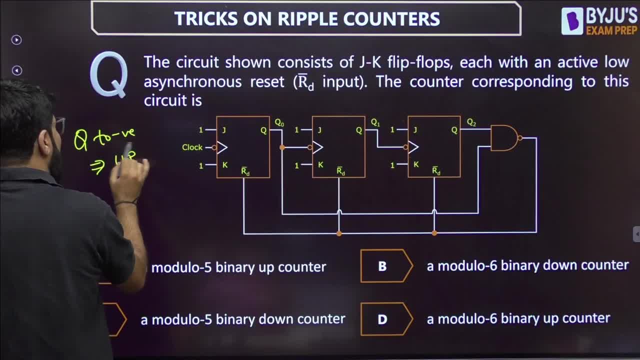 first: q to negative edge. q to negative edge, so it should be a up counter, or you can use the xor method also, so it should be up counter. it is not down. it is not down, okay. so what you have to now highlight, whether it is modulo 5 or modulo 6, usually it is three flip-flops, so it should be. 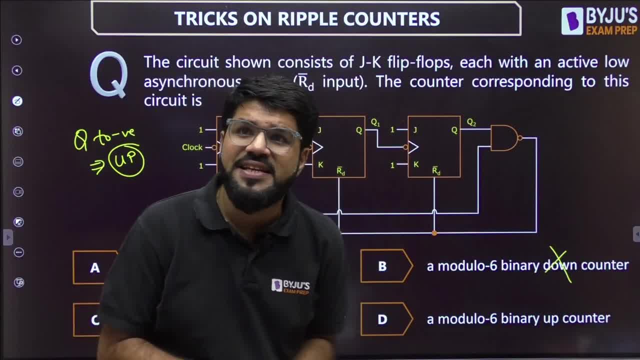 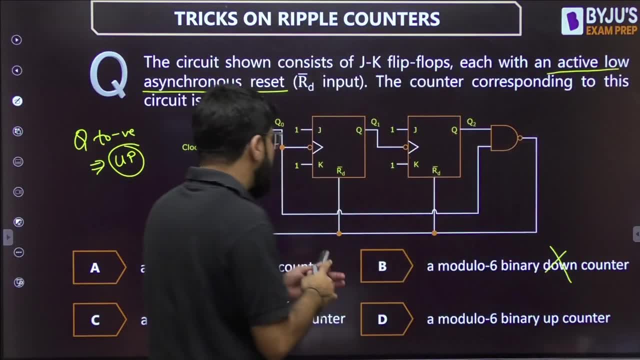 modulo 8. three flip-flops can count 2, power 3, that is 8 states. but this has a reset pin. now what is this? it is an asynchronous active low reset pin. what is active low? it is represented by symbol. also read bar. yeah, if they place bubble here, it means what? active low? what is the meaning of active? 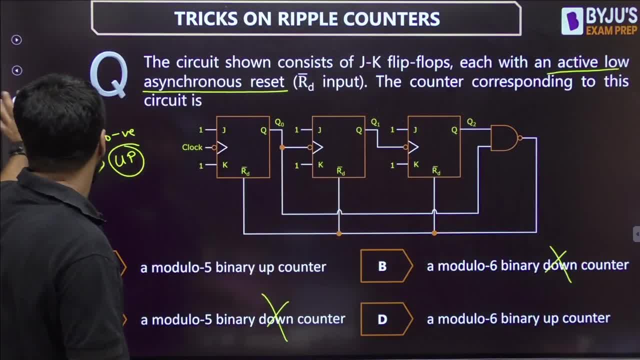 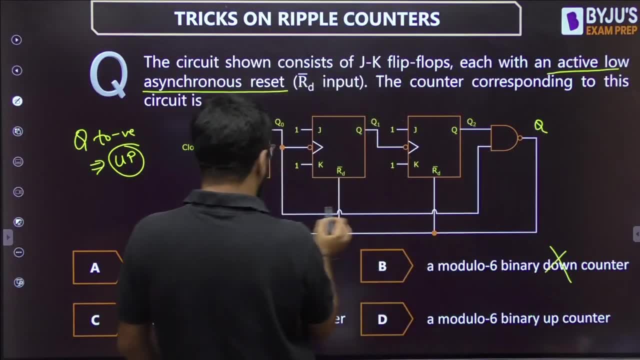 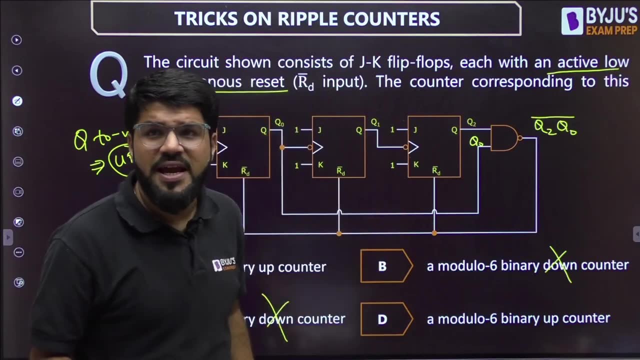 low. when you send a low signal here, then only the flip-flop will reset. then only the flip-flop will reset. now the signal is being derived from the output of nand gate. okay, input q2. and what is the input? q naught. okay, so q2, q naught whole bar. okay, the all the flip-flops will reset. okay, if the? 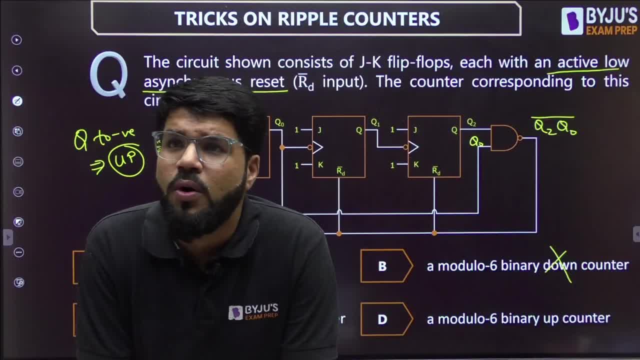 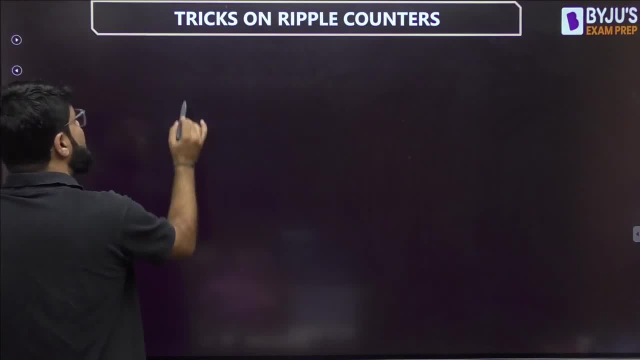 output of nand gate is zero. when is the output of nand gate zero? when both inputs are one one, when both the inputs are one one. so let me just write down what we have identified is that it is a up counter. let me try to write down the count sequence: q2, q1, q- naught, okay, because it is up. 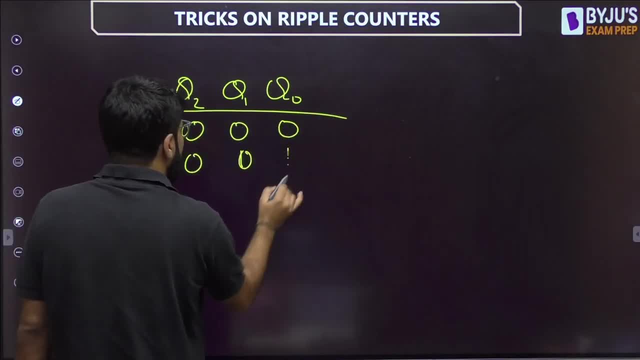 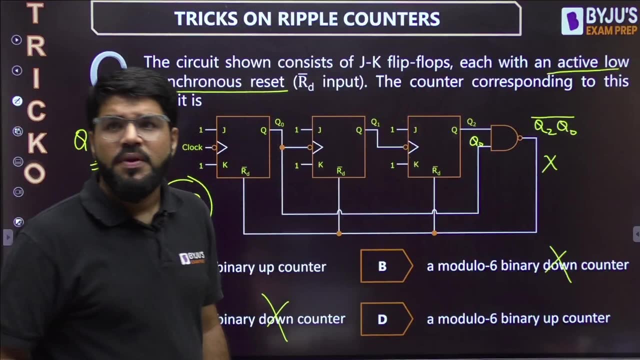 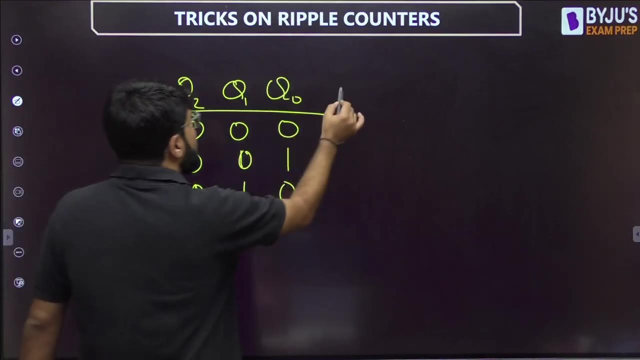 counter: zero, zero, zero, then zero, zero, one, then zero, one, zero. regularly. it should count like this, right. so the output of the nand gate is x. the output of the nand gate is x. okay, and i want x equal to 0. output of nand gate is 0. if both the inputs are one: right. if both the inputs are 1. 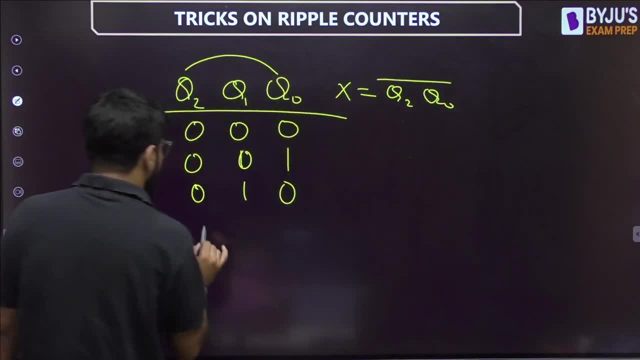 which input right, which input? q2 and q naught 2, q2, q naught whole bar. lena hai, both the inputs are not one zero, double one, then one zero zero, then i have one zero one, then i have one zero one. here we will pay attention. 1 0, 1, 1 0, 1 means x is equal to 0, because both the inputs q2, q, naught are. 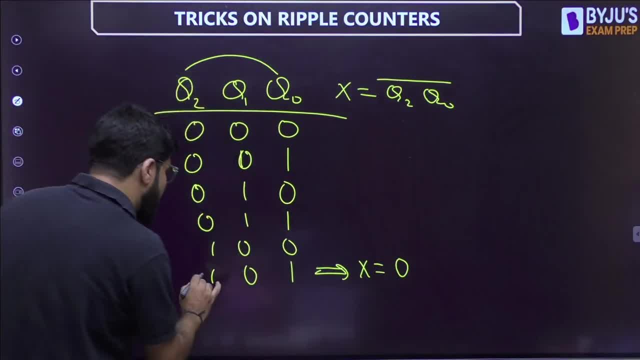 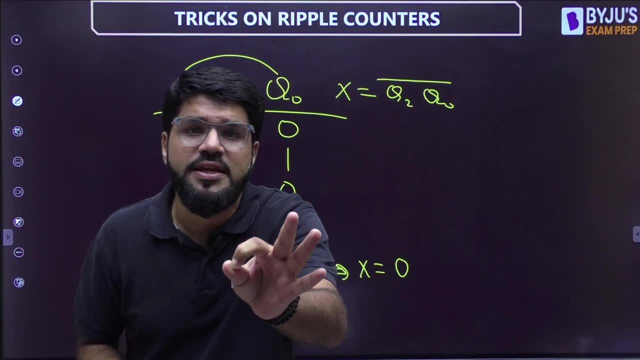 the flip flops will reset. okay, because all the flip flops will reset. so this state will not exist. actually, the state will be zero, zero, zero because it is a asynchronous reset. what is the meaning of asynchronous reset? pin right, it will reset the flip flop without waiting for clock. 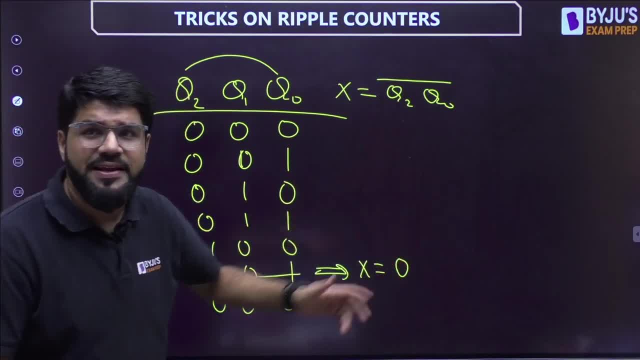 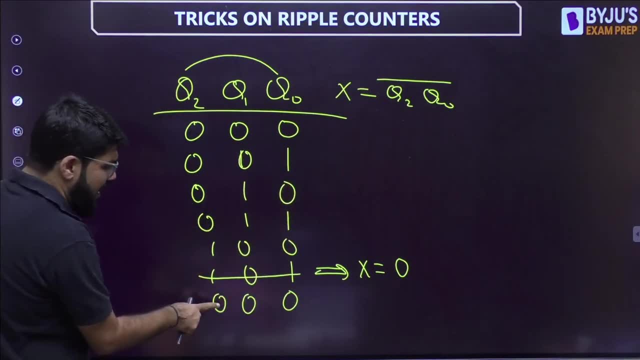 without waiting for clock, it will reset the flip flop almost immediately, in negligible time. that is why 101 state: but it goes away quickly, right? so actually the flip flop. next state, the counter next state is zero, zero, zero, right, which is actually a repetition. so how many states you?